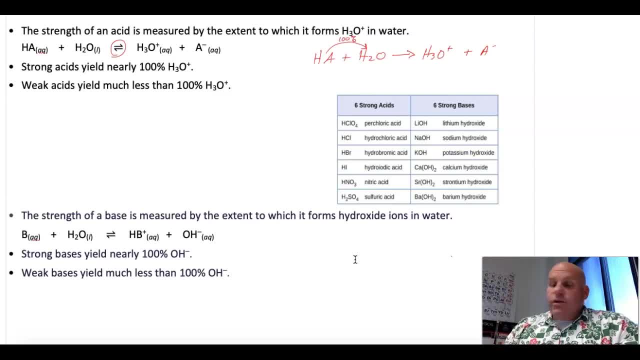 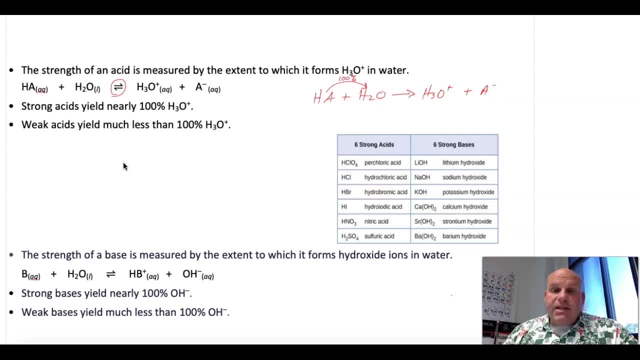 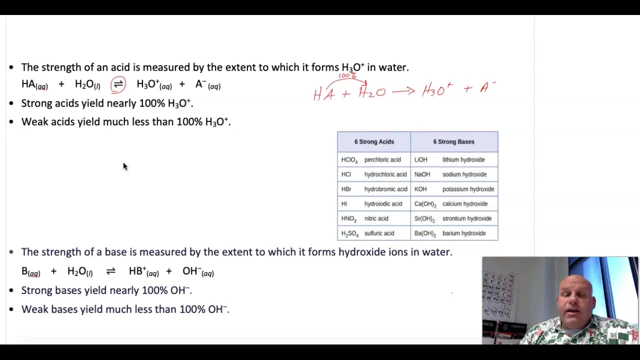 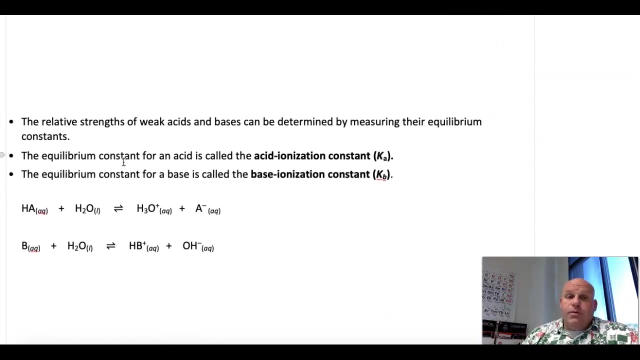 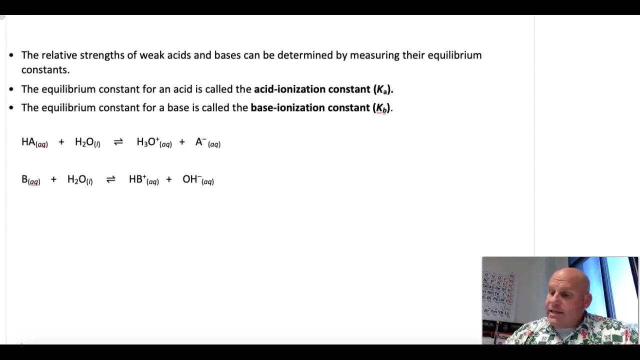 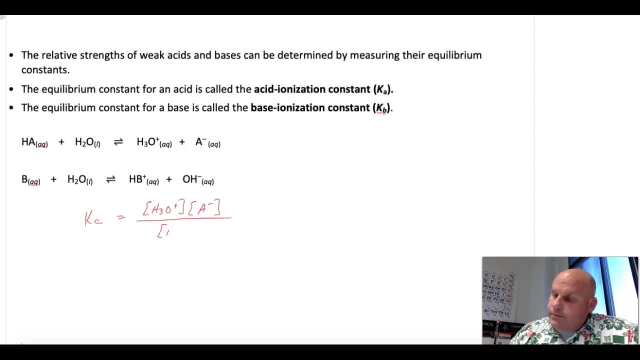 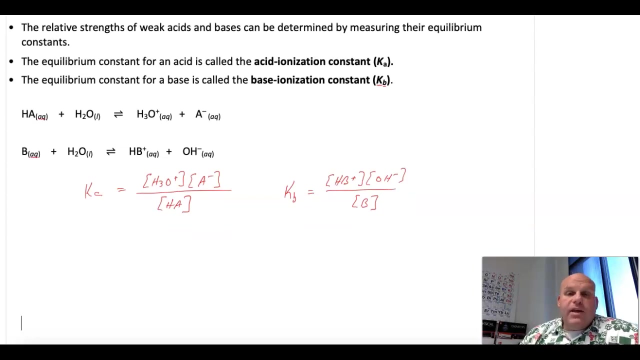 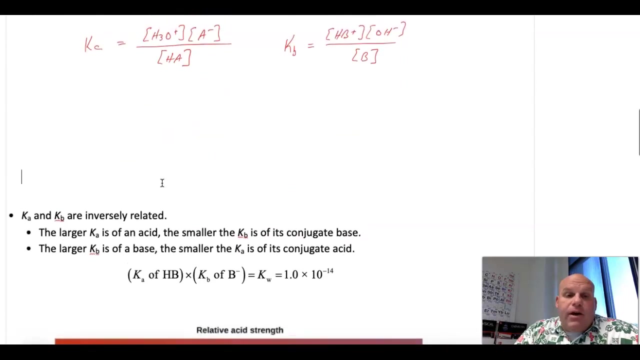 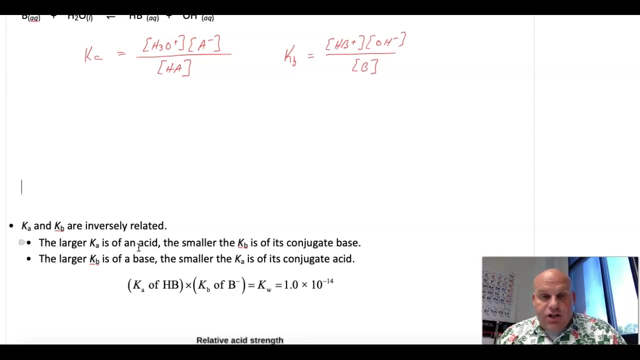 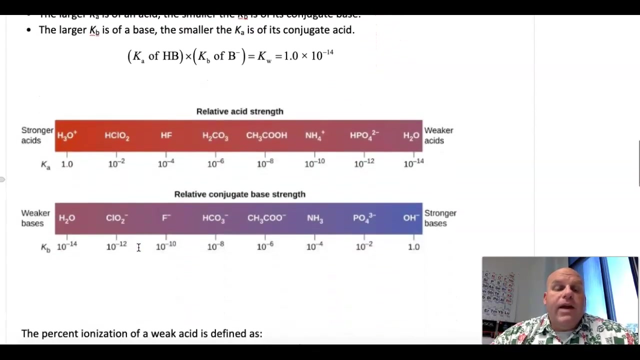 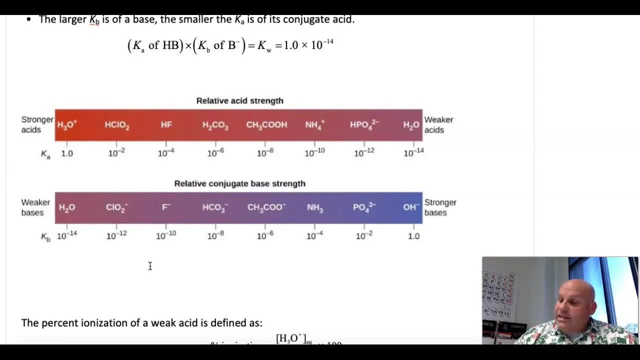 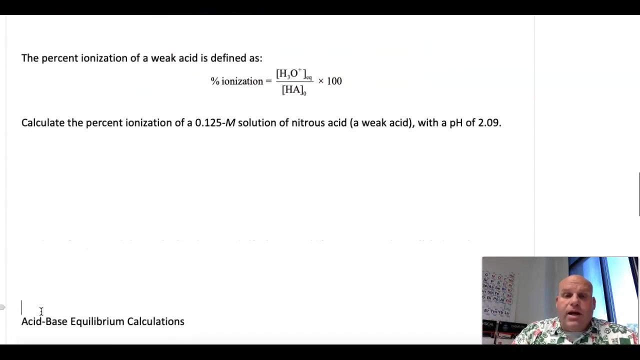 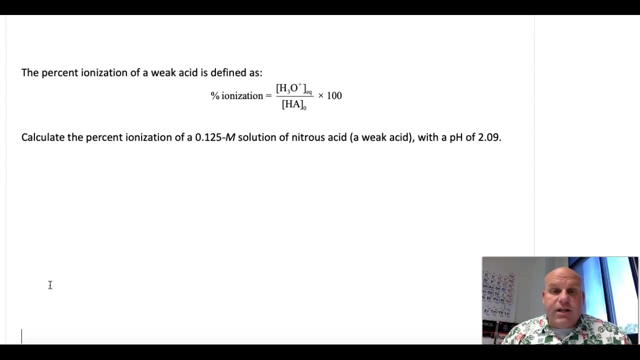 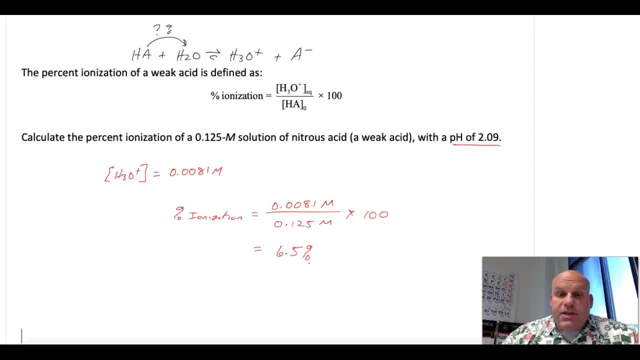 You're going to want to make sure you're comfortable with this, because this quick calculation, this quick percent ionization calculation, can actually help us in some future problems here in this section. avoid having to use the quadratic equation. Okay, let me say that again. Avoid having to use the quadratic equation from coming out of our last unit. I'm sure that that is music to your ears. 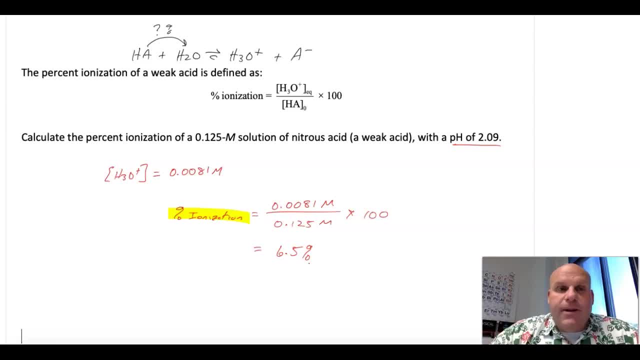 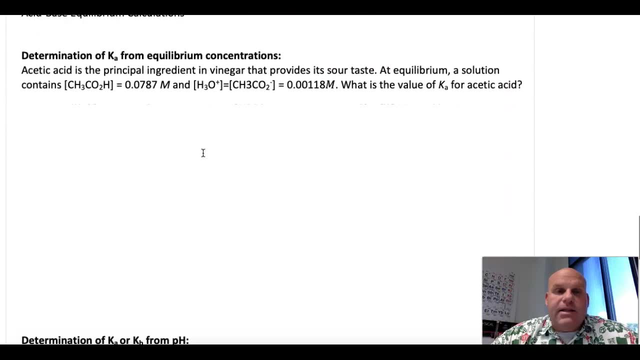 So I'll show you that. I'll show you that in some practice problems here in a minute. All right, we're going to finish off this section by looking at some different acid-base equilibrium calculations. acid-base equilibrium calculations. Okay, so here's our first type. 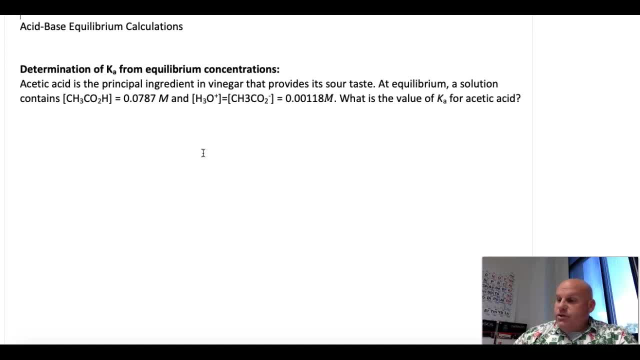 So we're going to determine the Ka from equilibrium concentration. So they will give us all of our equilibrium concentrations right in the problem. What is the value? Again, the question here is: what is the value of Ka for acetic acid? So I know that again, I can do that. 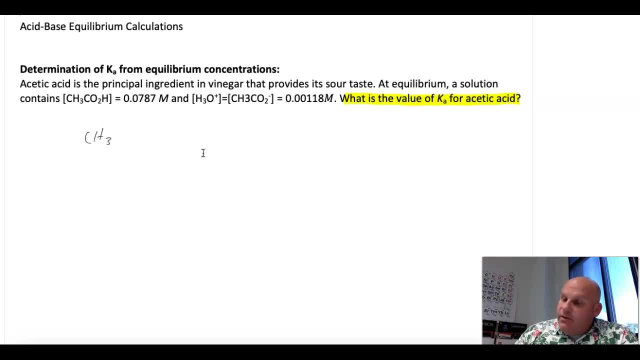 I can do that. I can do, since they give me the formula of the acetic acid here. maybe I already knew that or could come up with the formula there. I can do the specific reaction here, but I could also have just used the generic reaction for an acid reaction. 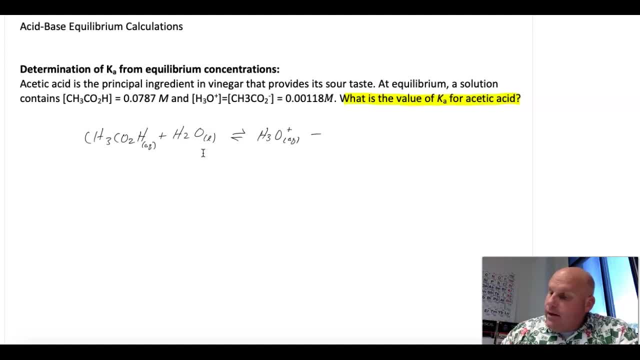 So either one works. It's not really that important, but I will go ahead and get my specific reaction here. Okay, and so they give me all of my concentrations. So my Ka is going to be the concentration of my H3O plus times the concentration of my acetate ion anion, here divided by my concentration of my acetic acid. 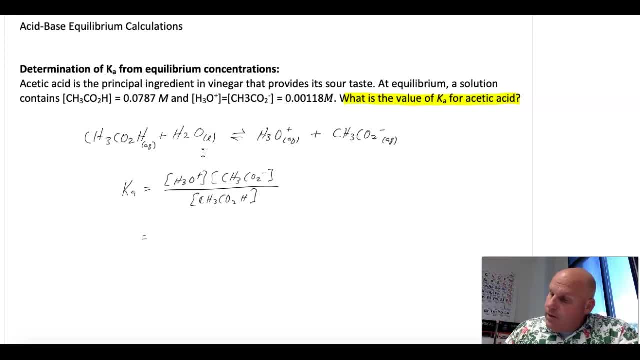 And again, they give us all those values in the problem. So I can just plug them all in and solve this out for my Ka values. Okay, so those are pretty simple, pretty straightforward. They give me all the concentrations. I just plug and chug and solve for my Ka. 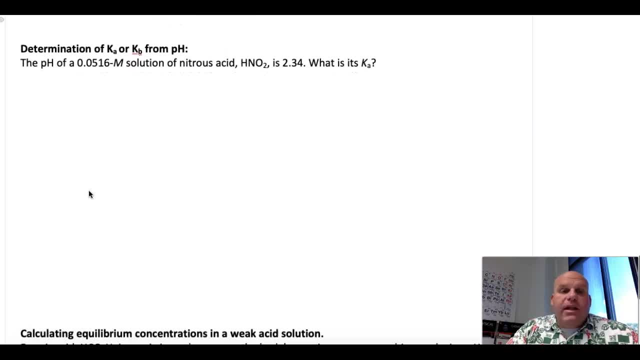 Okay, now let's Determine the Ka or Kb. Again, I'm going to do a Ka problem here. Kb obviously would be very, very similar, just talking about a base reaction instead from a given pH. Okay, so we got to think about what the pH tells us. 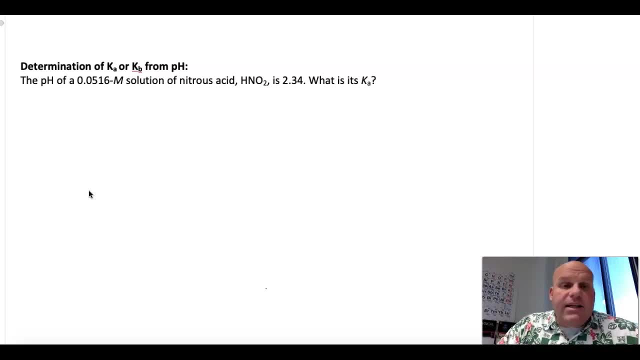 And in this circumstance, we are going to be utilizing our favorite ice tables again. So once again, let's come up with the reaction Again. since they went ahead and gave me the nitrous acid, I'll just go ahead and do my reaction with that nitrous acid. 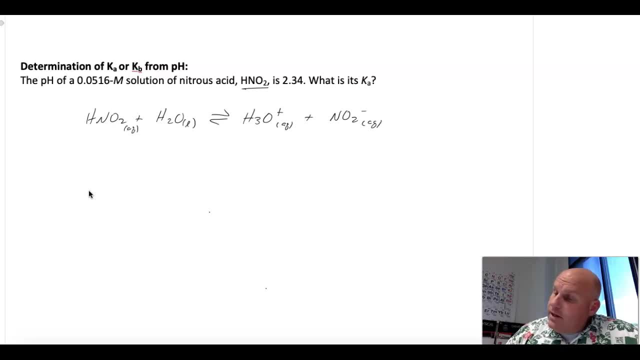 Okay, so we're determining the Ka again. Okay, so I know my expression. here is My expression for my Ka is going to be the concentration of H3O plus times the concentration of NO2, minus all over the concentration of my weak acid. 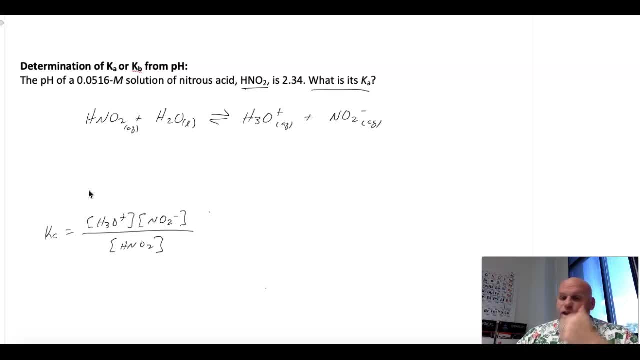 Okay, but unlike the last problem, I don't really have that information yet. So let's think about what I do have, and this is where our ICE table comes in. So I do have the concentration of our nitrous acid. so that's the 0.0516.. 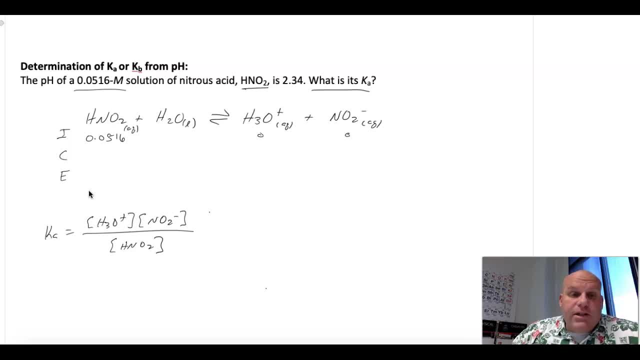 And again, my initial concentrations of my products here would be 0 and 0.. And, as we know, liquid doesn't matter here. Okay, and we can actually find, if I think about this, if I have a pH here that will allow me to find our equilibrium concentration of the H3O+. 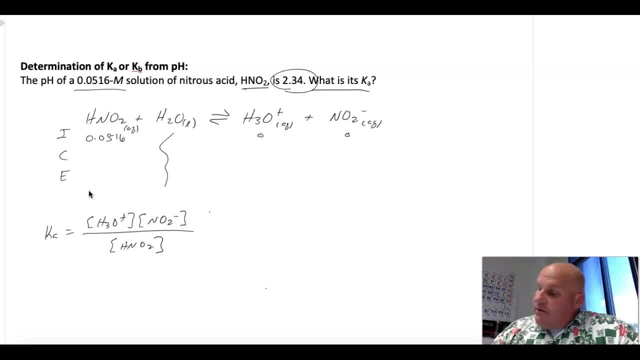 Okay so if I do the inverse log of this 2.34,, this pH of 2.34, I would get 0.. And I would get an H3O+ concentration of 0.00457.. Okay so, again, that is our equilibrium concentration of our H3O+. 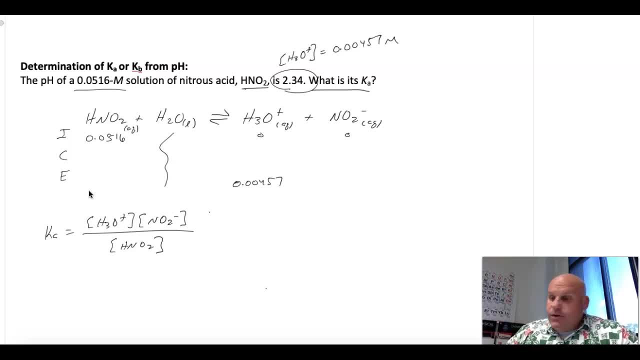 Okay, so now that fills in a lot of blanks for us. Okay, so, because of our stoichiometric relationship here, our concentration of our, our anion, is going to be the same. And now I know that my change here- because I started with 0, was this: 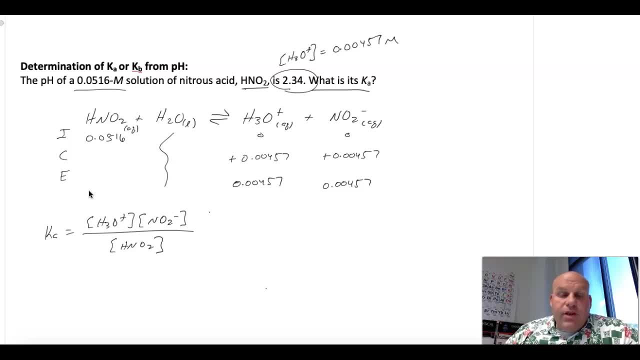 And once again, since our stoichiometric relationships are the same, I know that that means my change here is to lose that amount. So once I've done that, I can come up with the equilibrium expression or the equilibrium concentration of our acid as well. 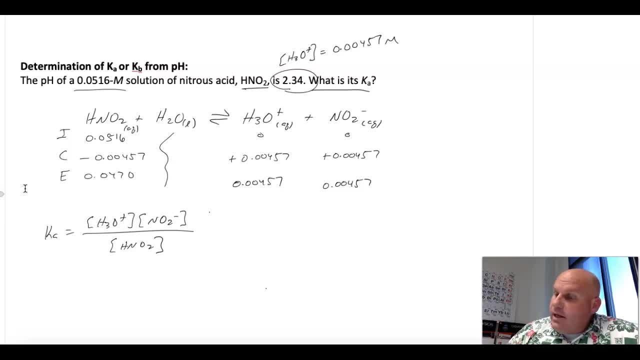 Okay, and now you'll see, I have all of those equilibrium expressions. I need to go ahead and solve for my Ka And I get a Ka value here of 4.97 times 10 to the number of 4.. Okay, how do you utilize an ice table there? 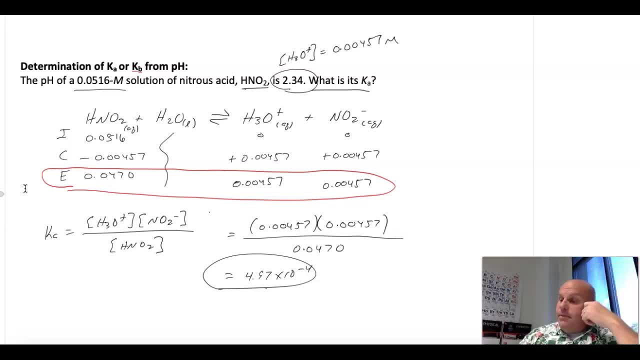 Because while I had the initial of the acid, I started with the other piece of important piece of information I had was the pH of of my solution. So that tells me the concentration of my H3O+. Okay, and then I was able to work, work my way through to get my equilibrium concentrations. 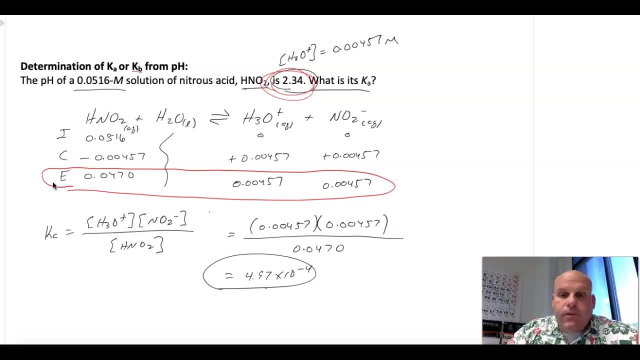 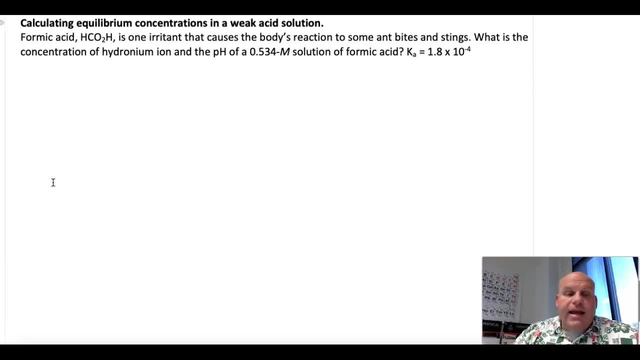 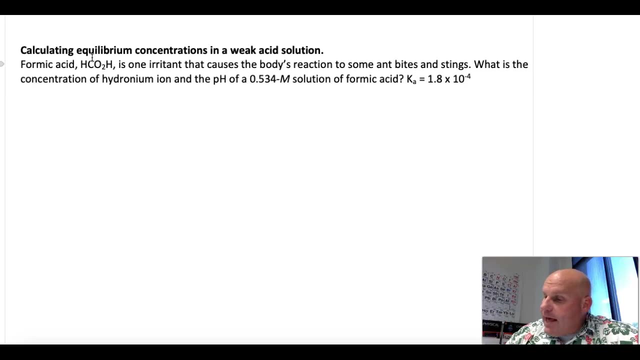 and then solve for my Ka. Okay, one more here. This is calculating equilibrium concentrations In a weak acid solution and basically, if I can, if I'm looking, trying to calculate my equilibrium concentrations, I'm often also going to be asked then to solve for the pH. 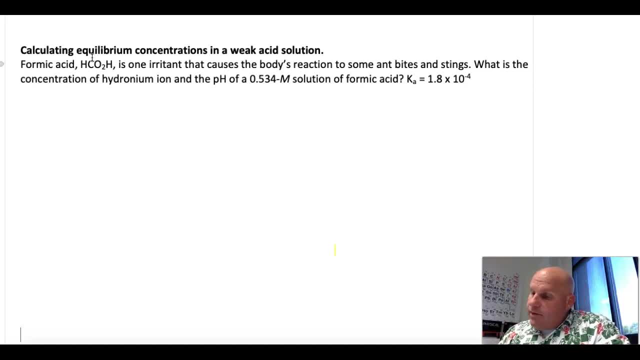 So right, because if I'm solving for my equilibrium concentrations, that means I'm going to be solving for the H3O plus concentration. So along with that, I'm also often going to be asked to identify the pH. Okay, so pretty common question there. 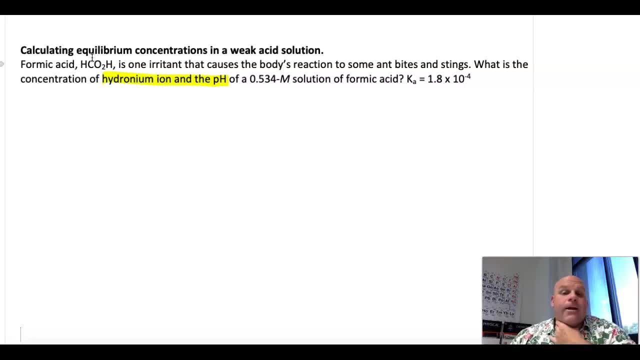 Okay. so this one has a little more to it, And this is where we can check our percent ionization, And if it's a certain below a certain value, we can- we can- avoid using the quadratic. So let me show you what that looks like here in a second. 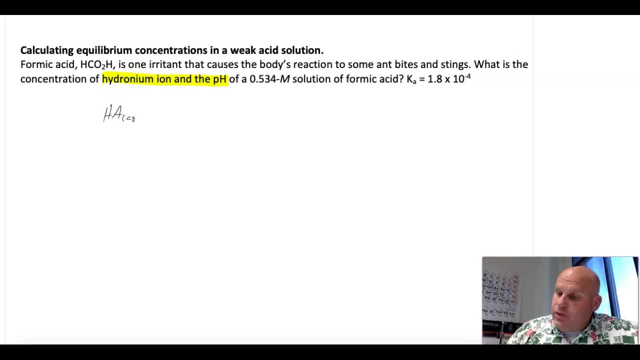 All right, so, as always, we'll do our reaction. This time I will just go ahead and use the generic acid reaction. Okay, and so now we think about what are what we have initially here. We know that we have an initial concentration of our formic acid, so of our weak acid. 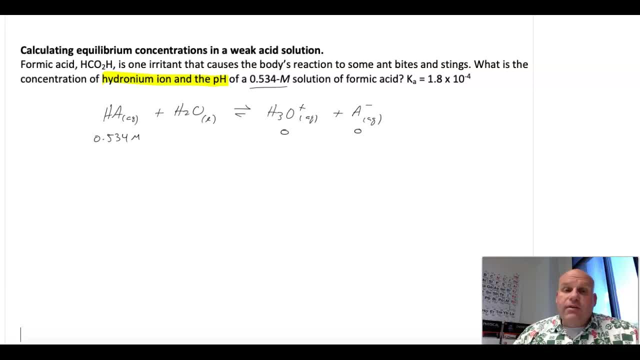 We know our initials over here are zero, but that's all the information we have. So there's nothing else about. there's no pH values here, There's no other concentration values here. So as I think about what we, the work we've done with ice tables, 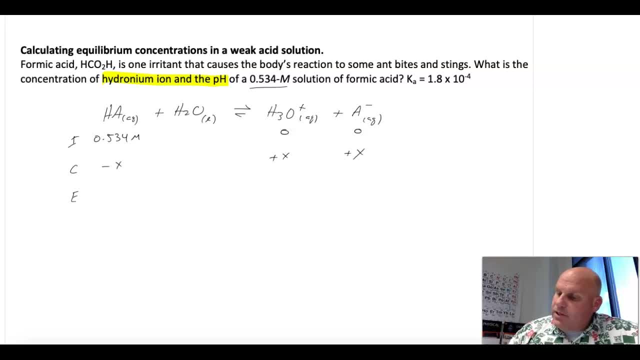 that's going to mean we're minus X plus X. So here are is our ice table. okay, We then know that the Ka is going to be the concentration of our H3O plus concentration of our A, minus times the concentration of our acid. 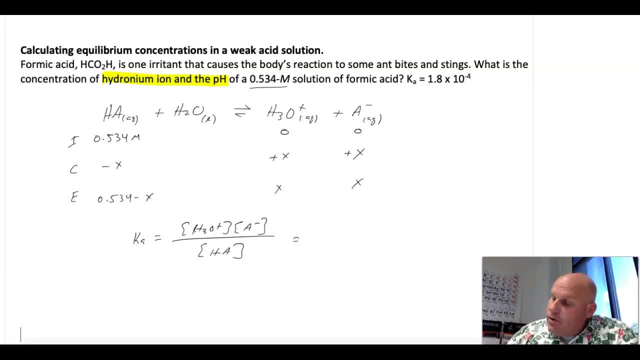 And we know these values are actually. let me just go ahead and rewrite it down here, since we know these values. Okay, And we know these values are actually, let me just go ahead and rewrite it down here. the Ka as well. 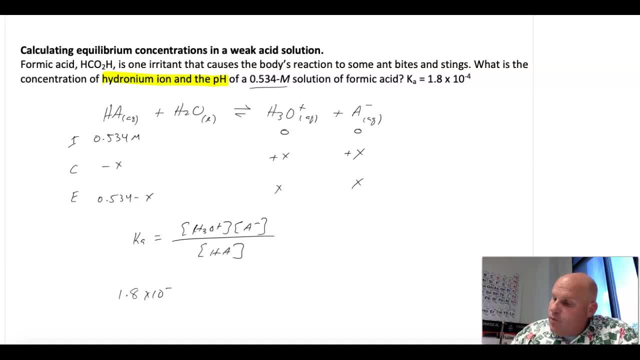 We know the Ka of 1.8 times 10 to the negative fourth is going to equal X times X over minus X. Okay, So there is an assumption that we can make here that if it's correct or valid, then we can avoid using the quadratic. 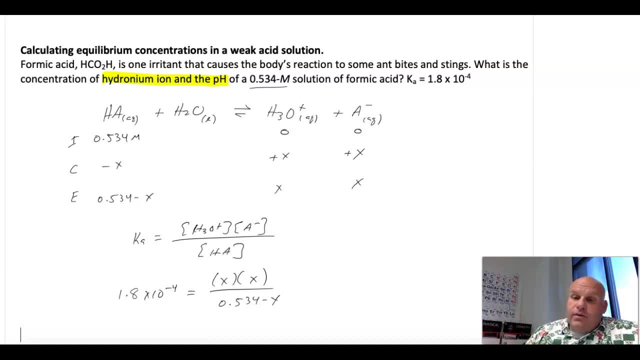 And that assumption is to say, because we are dealing with a weak acid, because we expect a low ionization, percent ionization, we can actually just go ahead and drop this x value off here and just make this value 0.534.. So what that does for me is it allows me to solve this out. 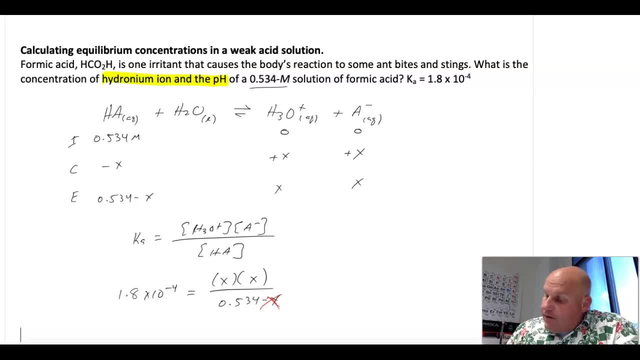 right. So now I can multiply 0.534 times the 1.8 times 10 to the negative 4th and I get 9.6 times 10 to the negative 5th equals x squared. Okay, let me go ahead and move up here. 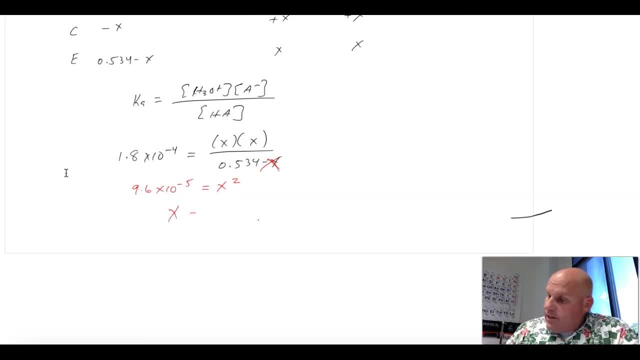 which then means that x is going to equal 0.0098.. Okay, if the assumption we just made, that that x, that amount of ionization, is going to be very small, less than 100%, we need it to be actually less than 5% to be able to solve this, So we can just go ahead and do that And then we can.